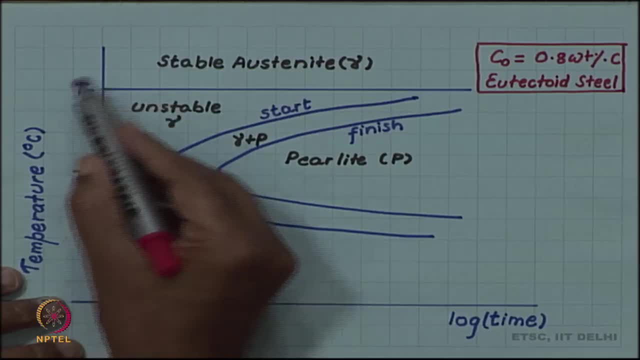 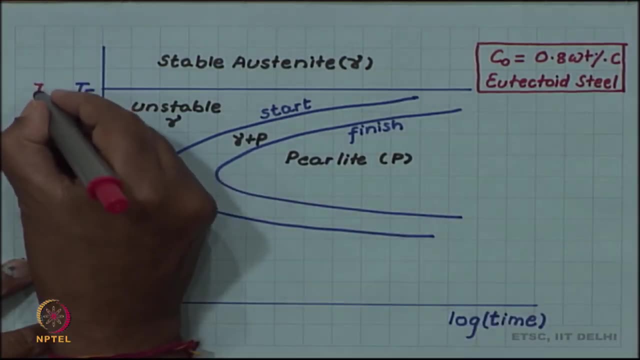 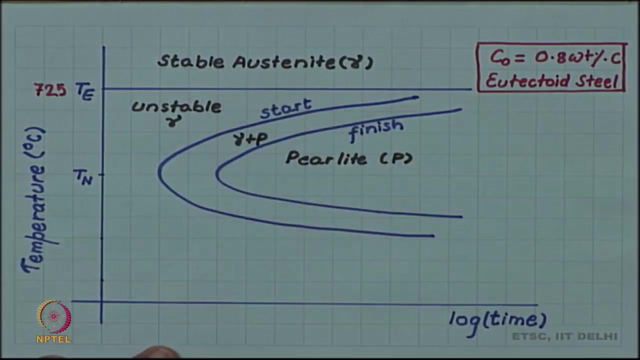 So this eutectoid temperature, T e is the transformation temperature for the eutectoid steel and that we know it is 725 degree Celsius. So that is the eutectoid temperature above which you have stable austenite. As soon as we cool it below that, austenite will be become unstable and 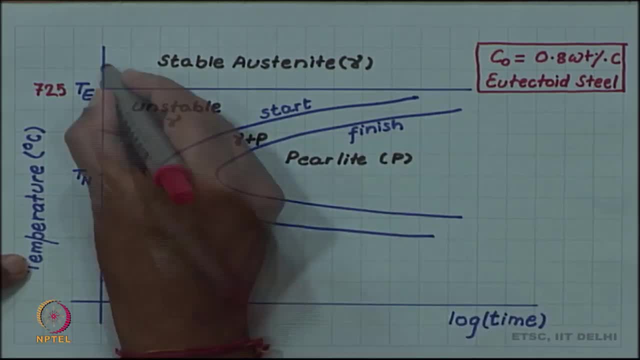 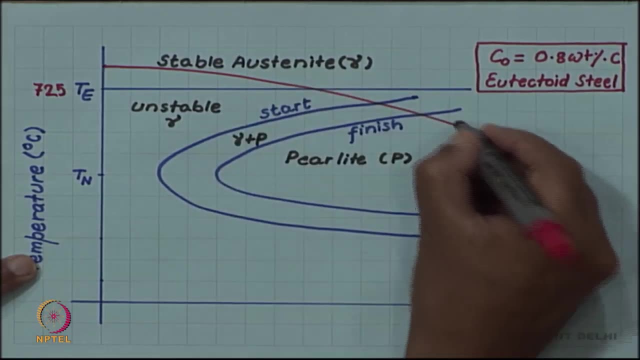 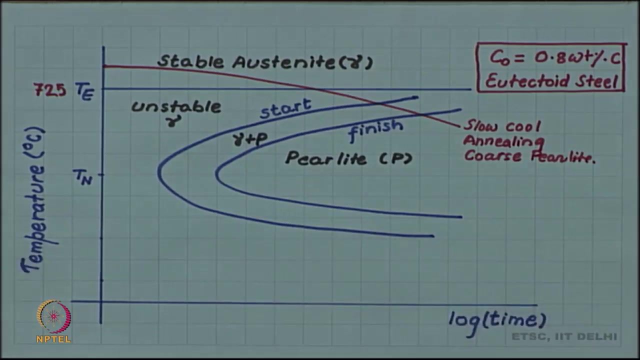 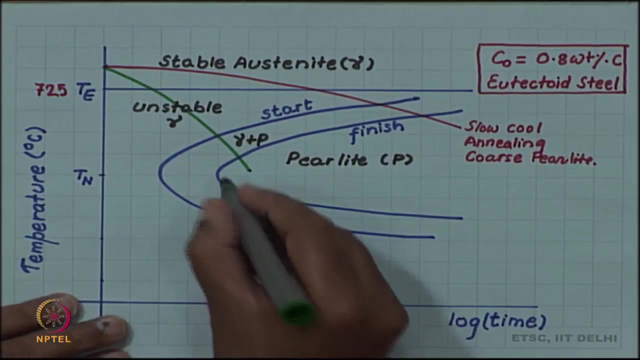 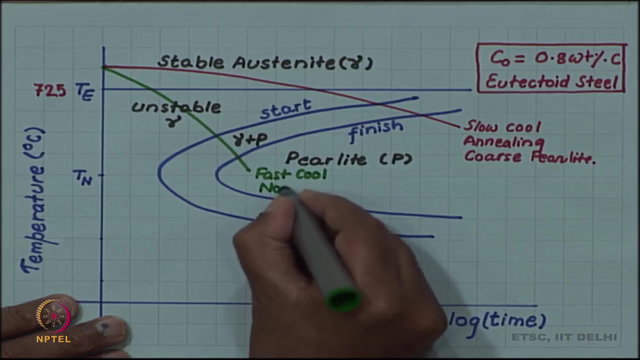 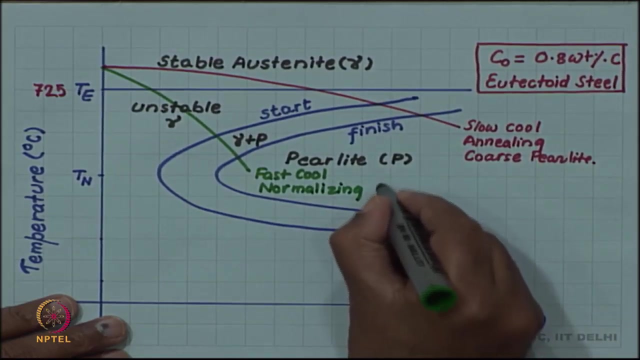 will start transforming. We saw two curves in the last video. one was for slow cooling, which was annealing- So this we call annealing- and this produced coarse pearlite. We had another curve- the faster curve, So let us call that fast cool- which was normalizing, and it produced fine pearlite. for us, The 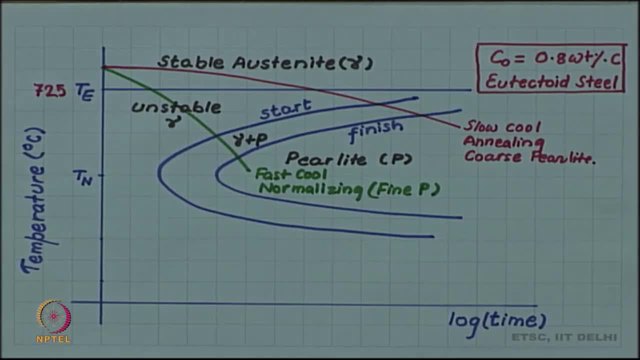 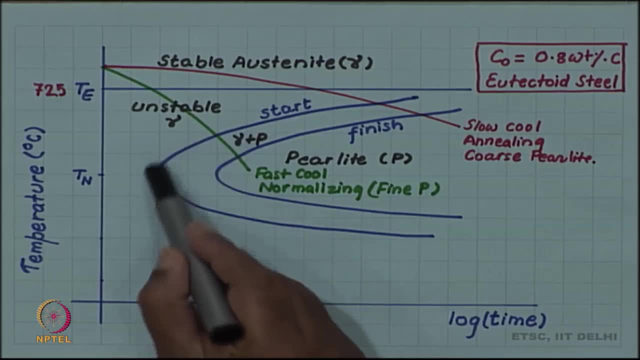 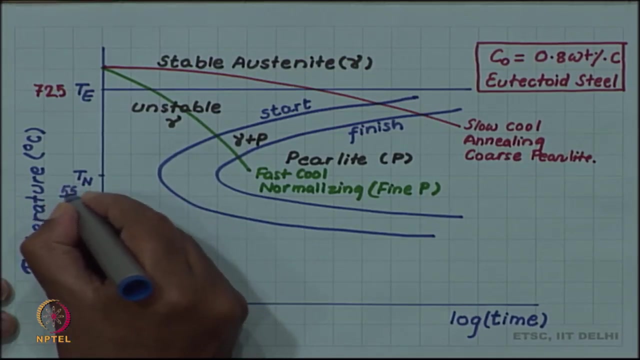 question now is if we cool extremely fast, so fast that we miss the nose. this is called the nose. So let us say, of the C curve where you have the fastest transformation rate. the temperature corresponding to that I have marked as T n. that temperature is about 550 degree Celsius. 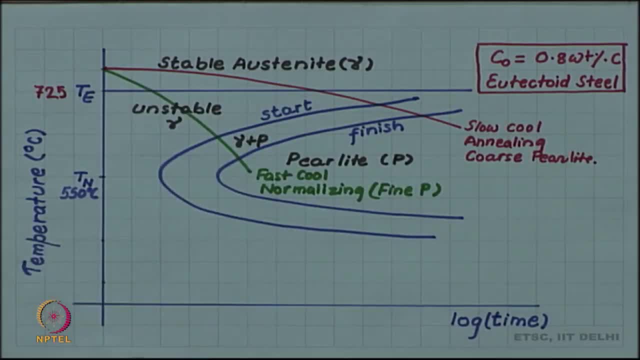 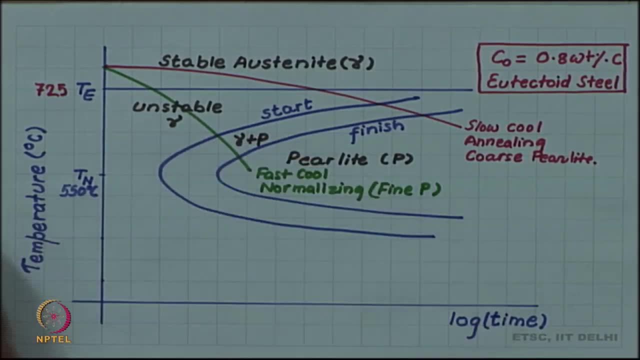 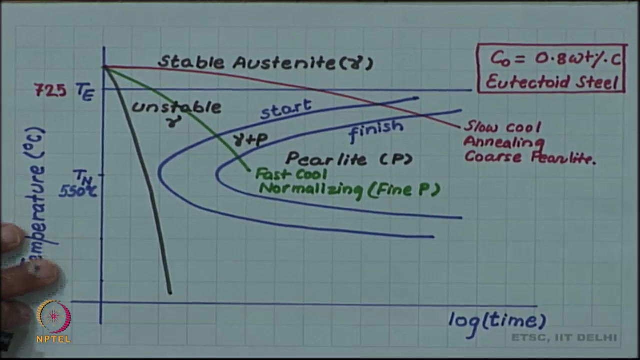 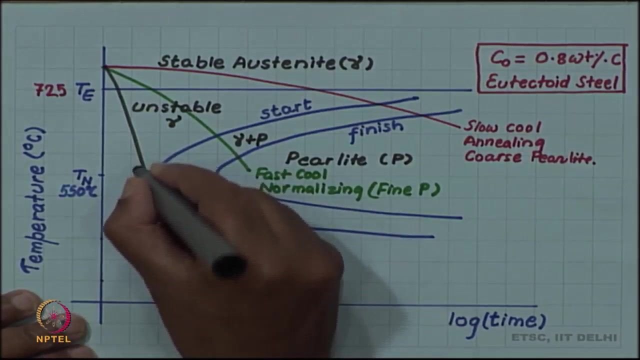 If you start cooling faster and faster, then you may achieve a cooling rate, an extremely fast cooling rate. Let us say So I have represented by this line that I miss the nose of the C curve extremely fast cool. This is what is called this kind of treatment which gives you extremely fast cooling. 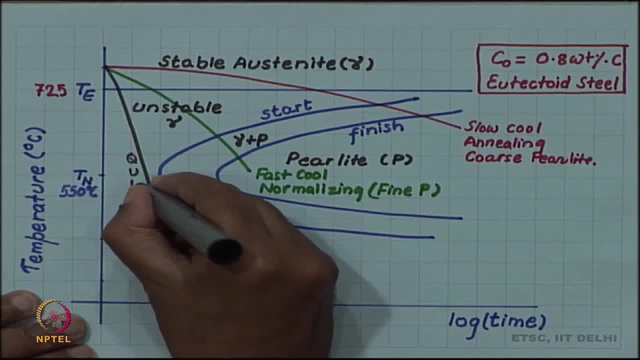 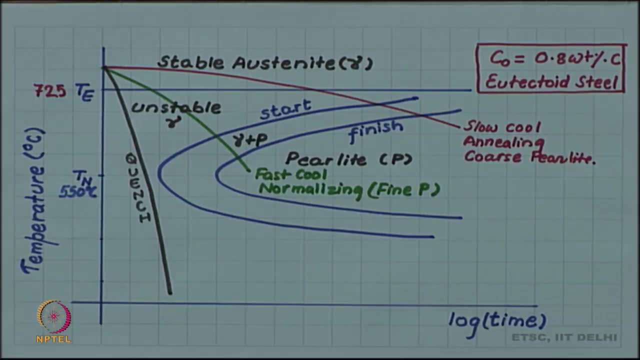 is called quenching. So I am quenching the steel now. So if you quench the steel, if you cool it very fast, So if you take it out from the furnace and drop it in water- cold water kept at room- 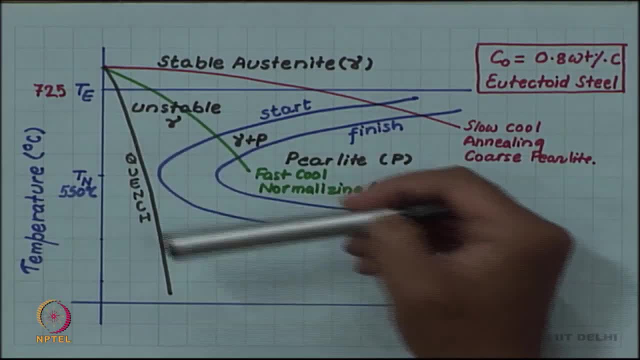 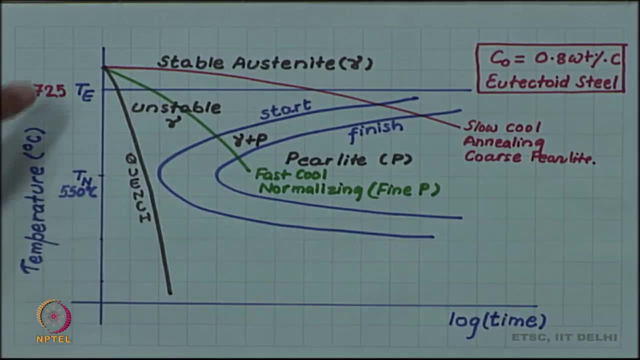 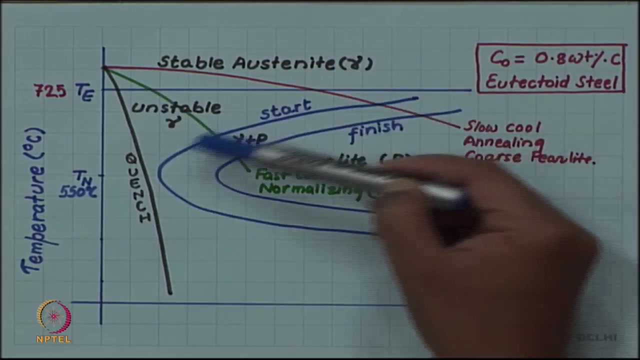 temperature. So then the cooling is very effective in water and you have a very fast cooling rate, and that is called quenching. So what would happen? What will be the fate of this austenite which is being cooled so fast that you are missing even the start curve? 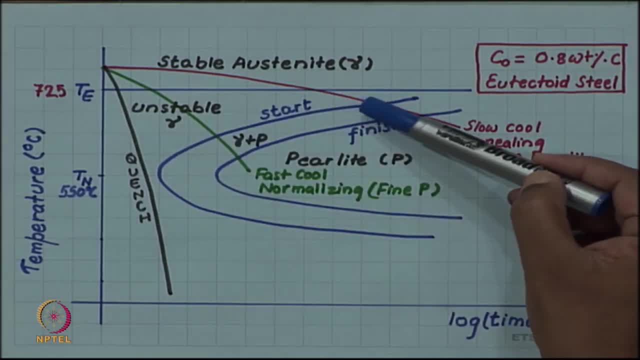 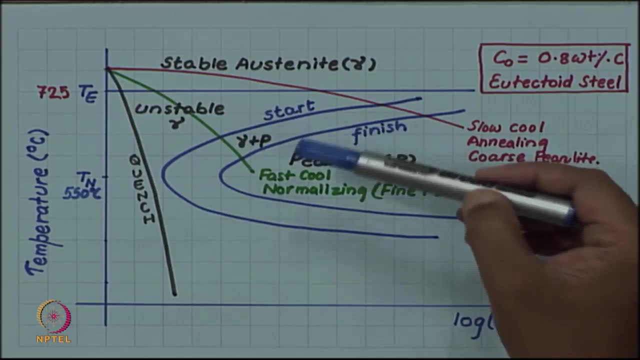 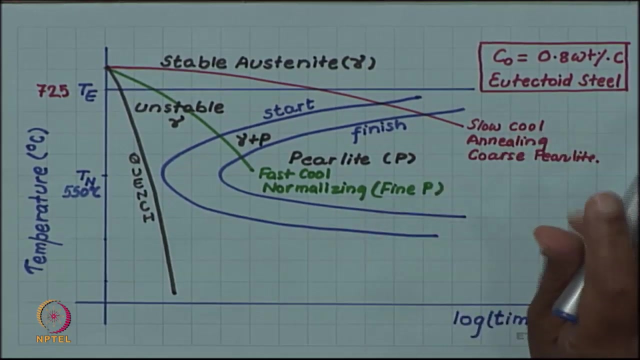 So obviously there will be no pearlite formation in this. So this cooling rate, because you are not even hitting the start curve for the pearlite transformation. Recall, we had a similar situation in liquid to solid transformation where we had C curves for start of crystallization and finish of crystallization. So there also. 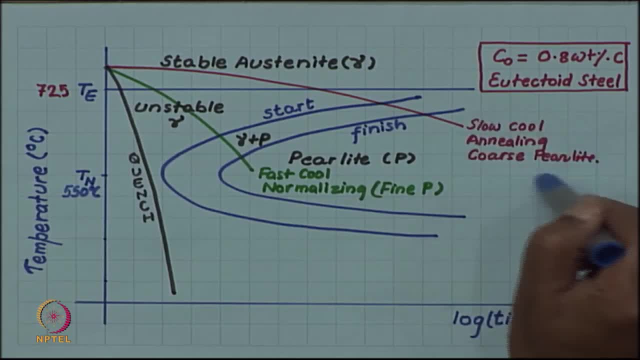 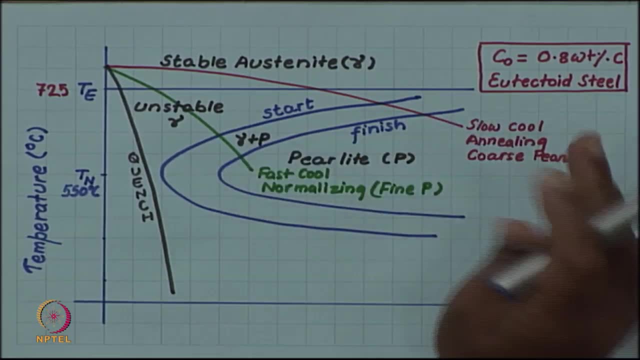 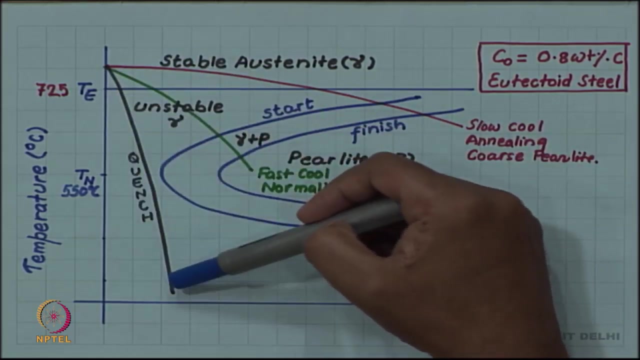 if we cooled slowly, we got coarse grains and we cooled faster, we got fine grains, So we got fine grains. So these situations are analogous to the liquid, to solid transformation, and there, when we quenched so fast, if we cool the liquid so fast that it missed the nose, 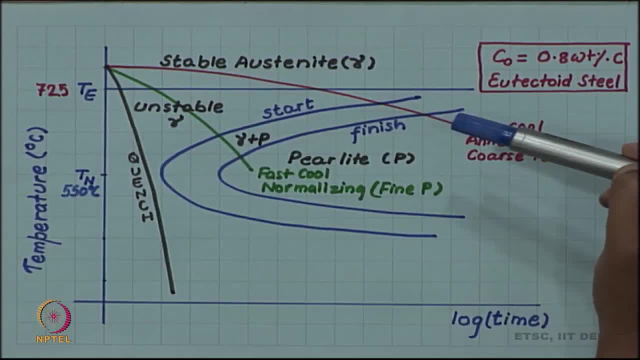 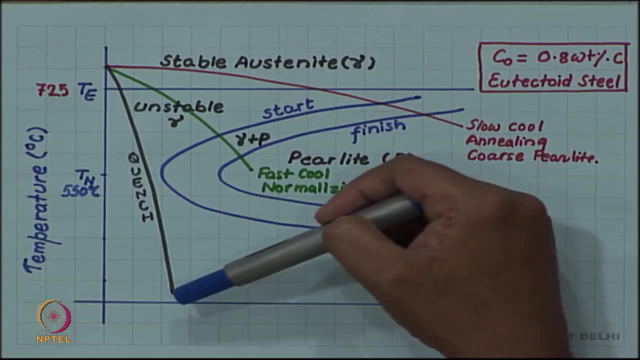 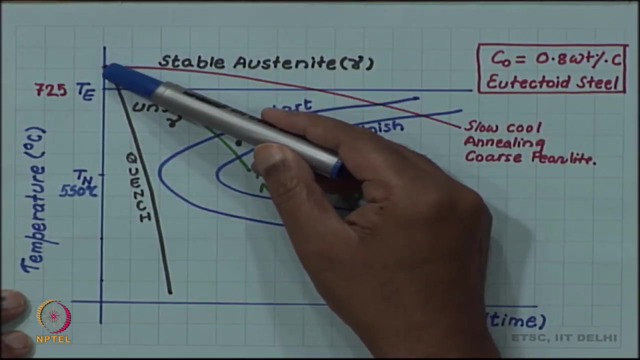 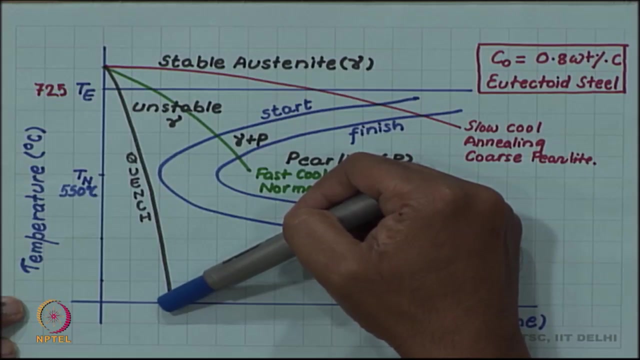 of the C curve in the liquid to solid transformation. Then we retained the liquid structure right down to the room temperature and that was super cool liquid or glass. So one possibility was that if we cool austenite very fast, Do we retain this high temperature phase? Do we retain this austenite down to room temperature? 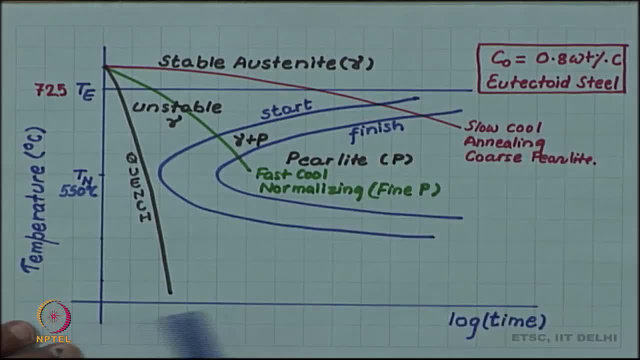 down to low temperatures. However, in the case of austenite, this does not happen. nature throws another surprise at us, and that is what is called the martensitic transformation. So what really happens here is that at some transformation, at some temperature. So we 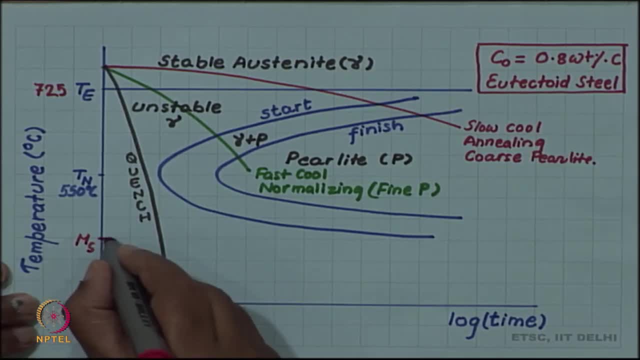 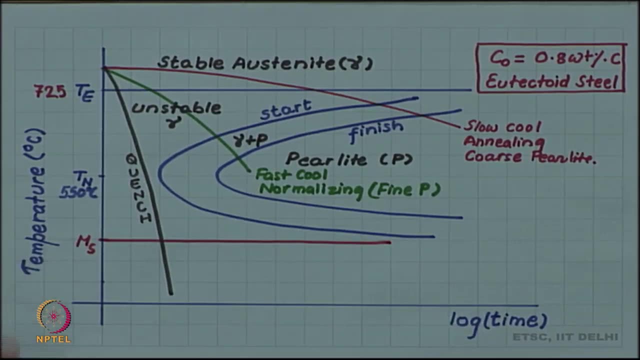 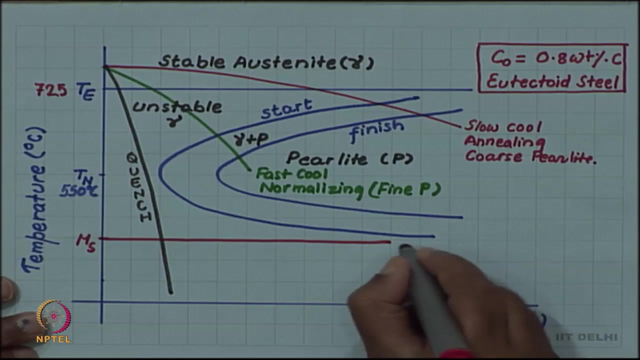 have a new transformation here. let me label it M? S. when I draw a horizontal line here, a new transformation begins and that is called a martensitic transformation. So M? S is the start of the martensitic transformation. M? S- martensitic transformation. So this is: 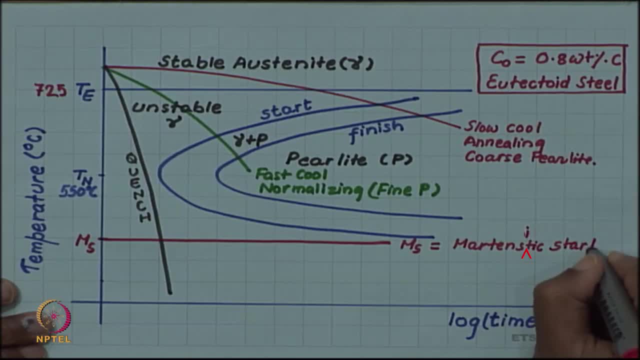 the start. let me call it: this is the temperature at which martensitic transformation begins. and then there is another temperature below that and I draw another horizontal line there which is M F, which is finish of the martensitic transformation. So martensitic start temperature and martensitic finish temperature, so as the steel is being 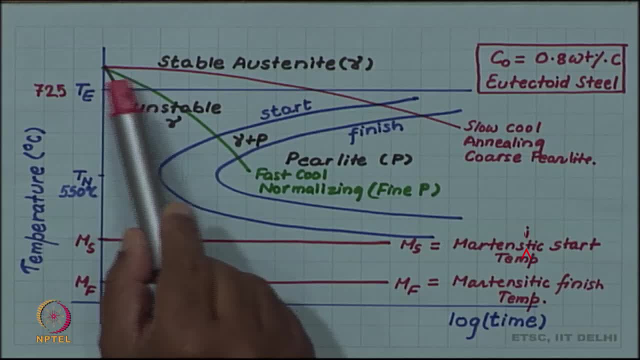 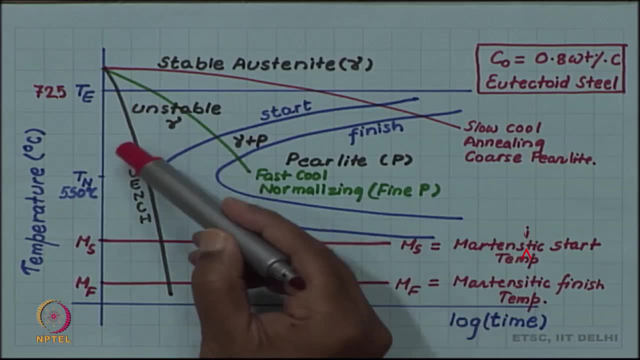 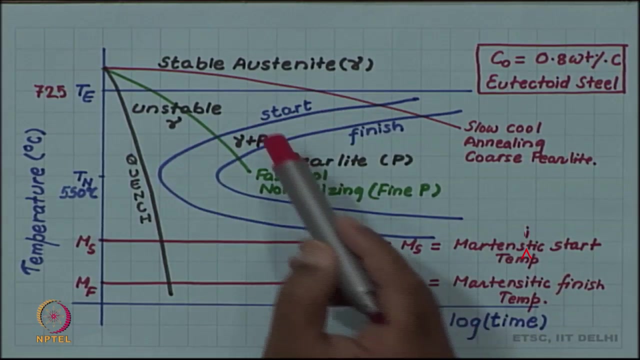 quenched. as we cool below T e, it will change from being stable to unstable austenite. That unstable austenite will is being cooled and is never able to transform to pearlite. because you are missing the start of the pearlite transformation. 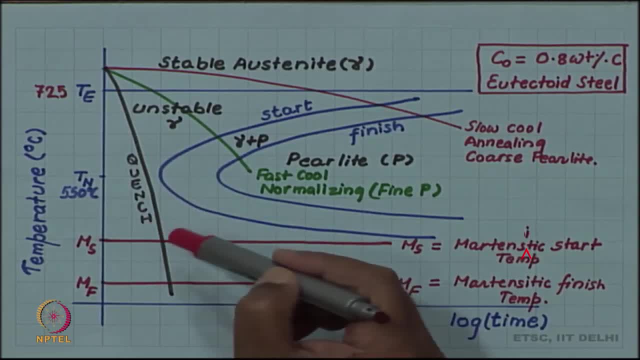 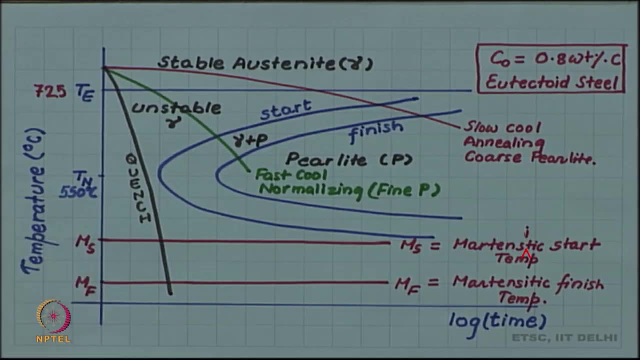 And then it is becoming more and more unstable and finally, when it crosses M s, it is starts transforming into a new phase called martensite. so we can write here the phase as austenite plus martensite. I am using M for martensite, and then below M f you will have martensite. 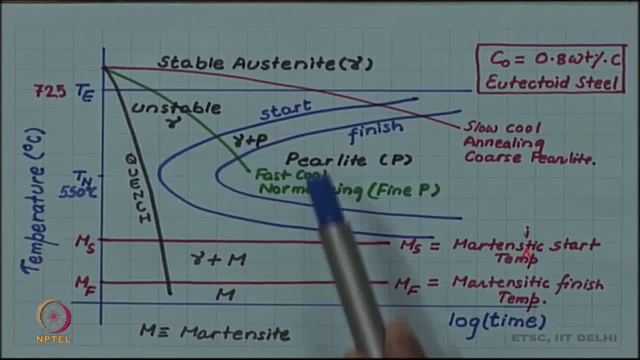 One difference you are immediately seen between the pearlite transformation and the martensite transformation, And that difference is that although for pearlite transformation I was having c curve, for martensite transformation I am having horizontal line. This is because in martensitic transformation the amount transformed 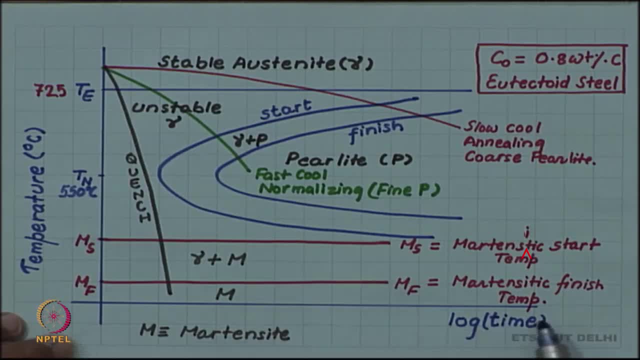 is independent of time. Now, although our x axis is, time plays no role in the transformation of martensite, So amount of martensite transformed depends only on temperature. So at m s the transformation has just begin, So a very small amount of austenite has transformed. 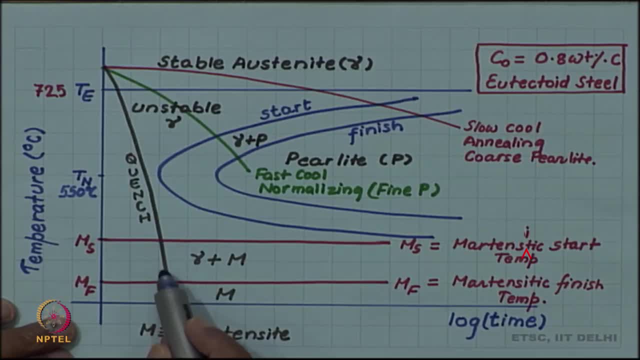 into martensite. as we cool further, more and more amount will transform and finally at m f we will have 100 percent martensite. So in between m s and m f we can think of, let us say, at some temperature we will have 50 percent martensite. So gradually the amount. 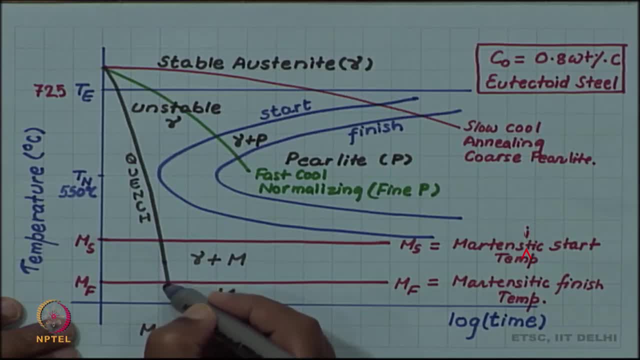 of martensite will change as we lower the temperature. So But the transformation rate itself is very, very fast, such that as soon as we reach those temperatures, within no time the transformation is completed to martensite. And if we hold at that temperature in between temperature, let us say at 50 percent martensite, if we 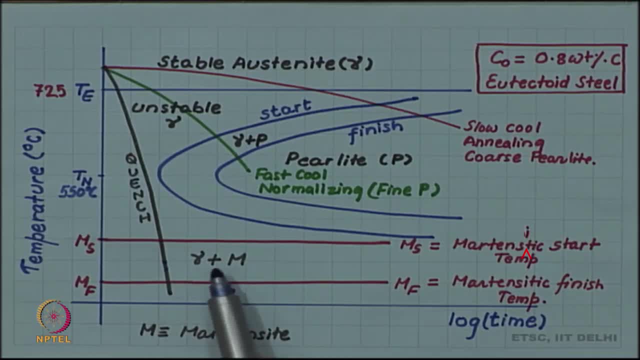 allow more time, then the amount of martensite is not going to increase. it is going to remain 50 percent as the time passes. So the role of time disappears in the transformation of martensite is a very fast transformation and the amount transformed depends only on the temperature. 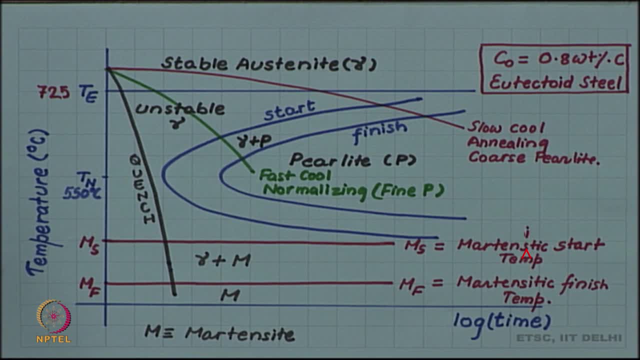 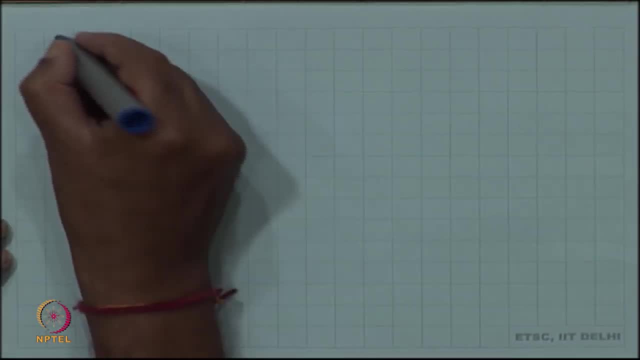 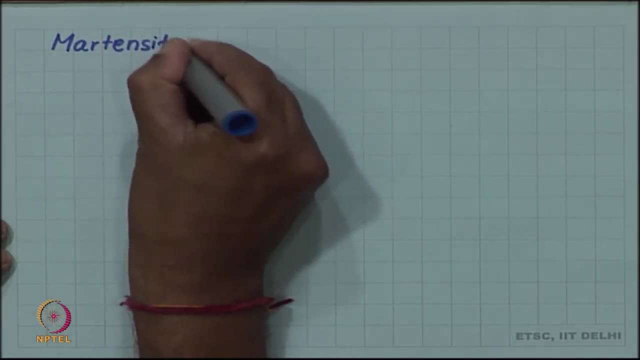 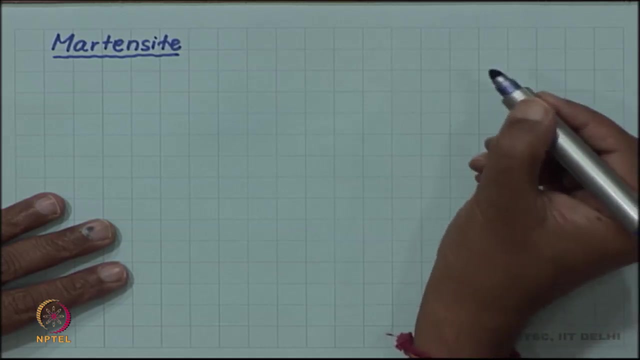 Let us look at this martensite phase. although we are saying that a martensite phase is formed, we have not described what this phase is. So let us look at what this martensite phase means. So this phase we have not seen in the iron carbon equilibrium diagram. So, first of all, 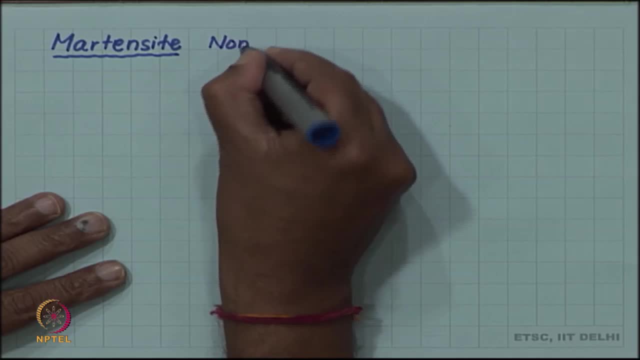 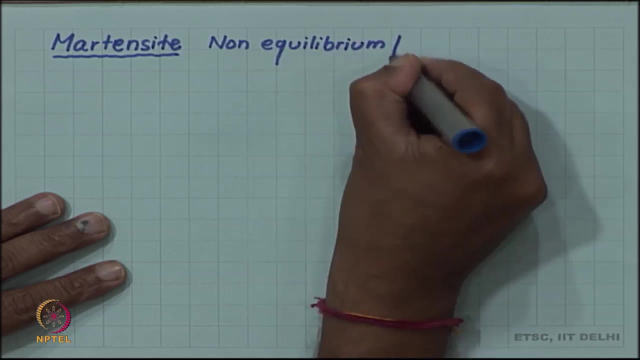 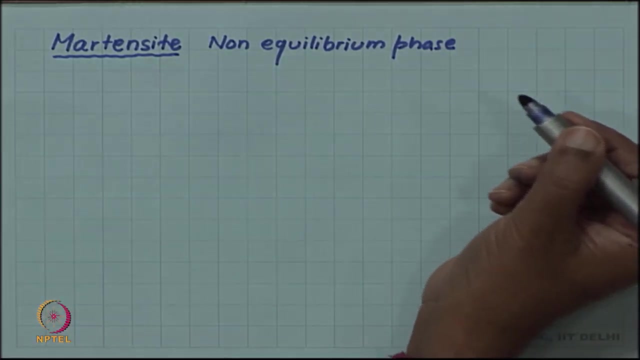 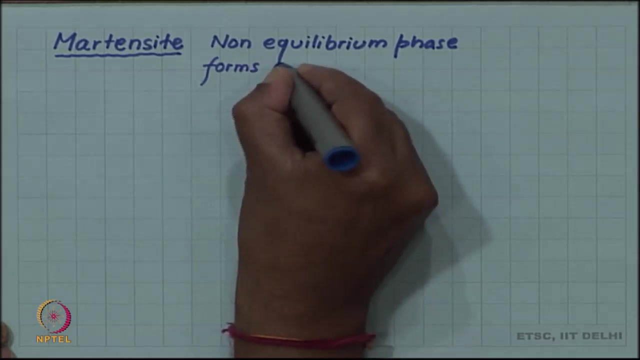 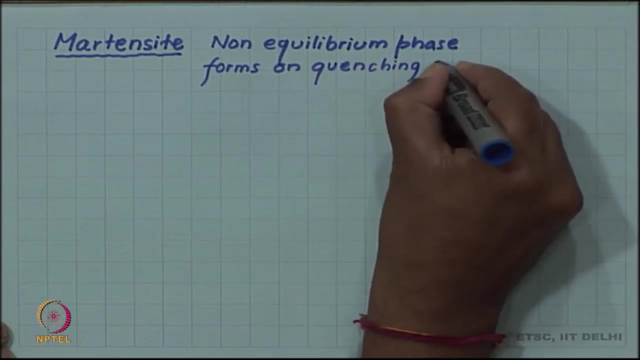 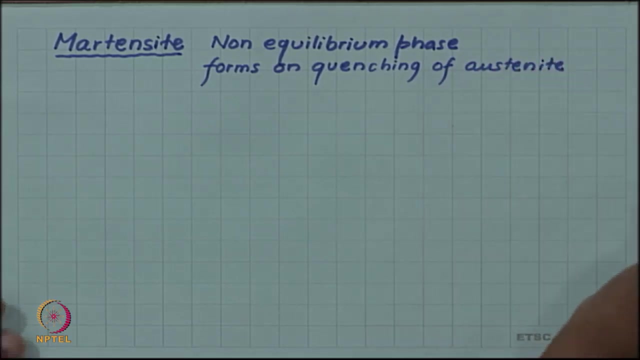 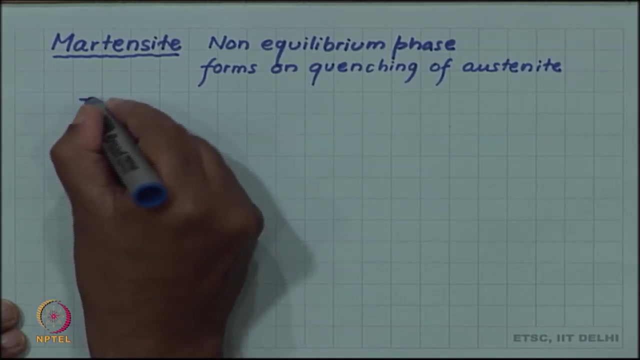 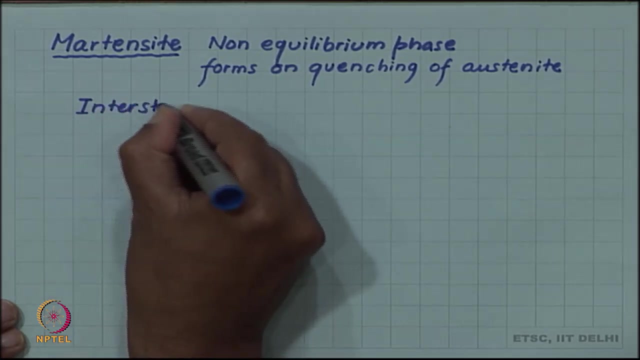 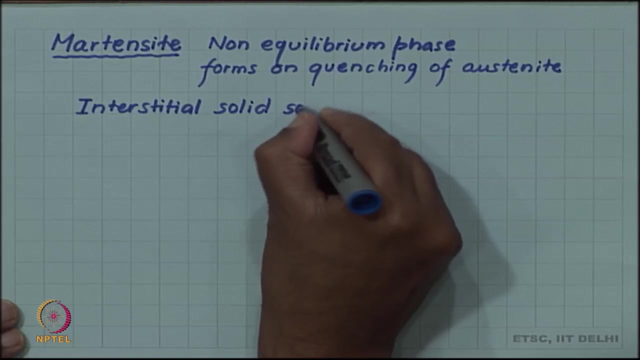 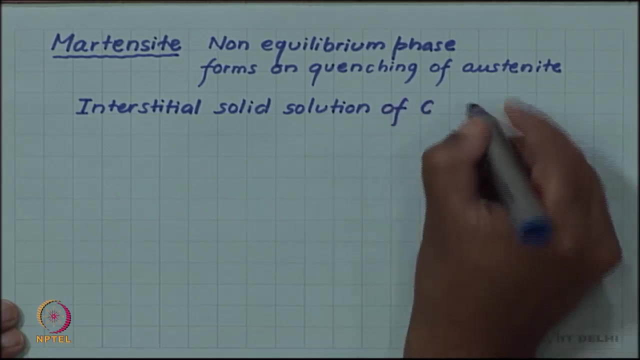 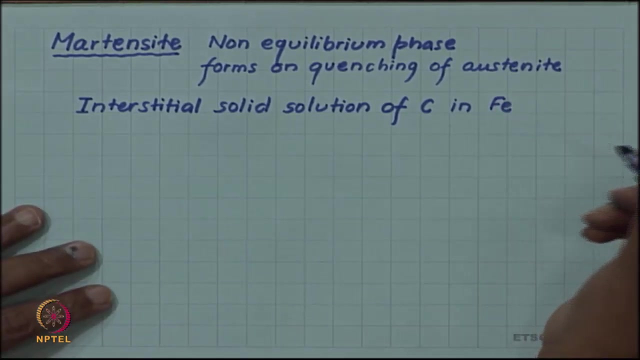 it is a non-equilibrium phase and it is formed on extremely fast cooling of austenite, So quenching of austenite or extremely fast cooling. We can define martensite as an interstitial solid solution Of carbon in iron. So this is same as austenite or ferrite, only the crystal structure now is 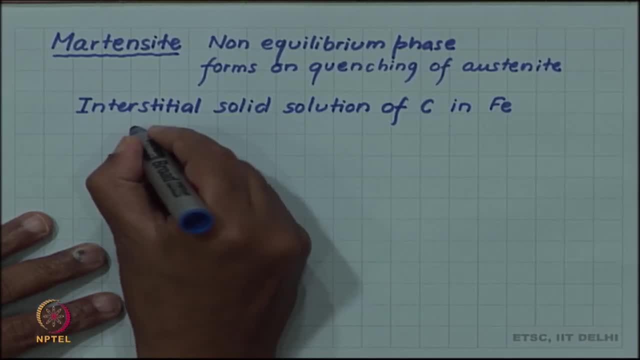 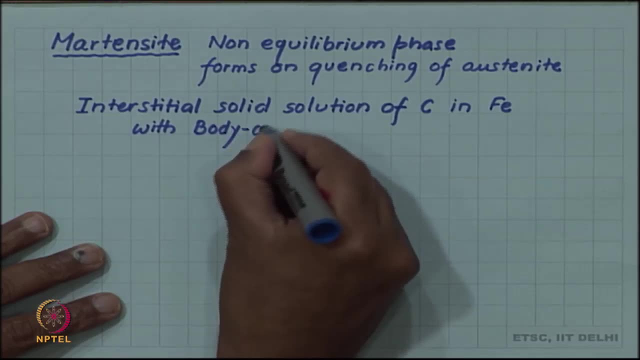 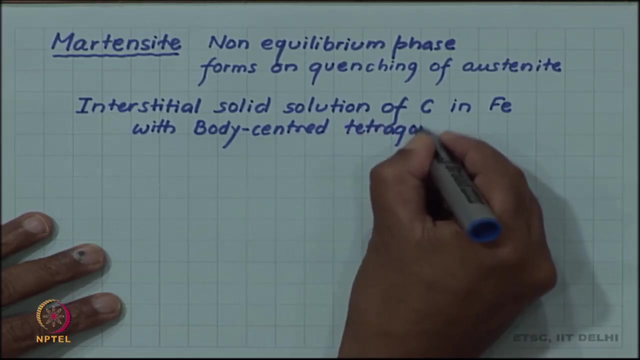 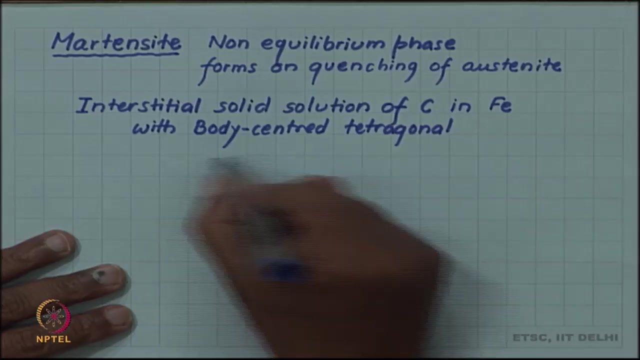 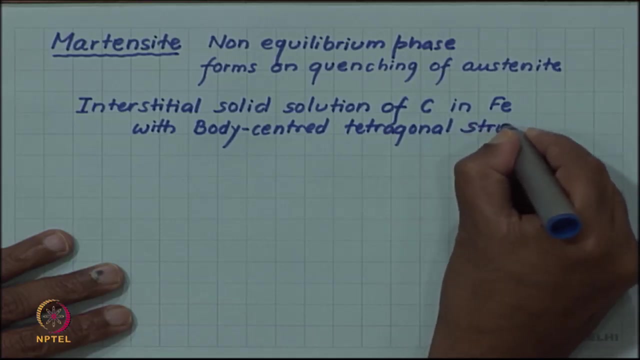 different. So the interstitial solid solution of carbon in iron with body centered tetragonal. So both ferrite and austenite were cubic phases, but now we have a tetragonal structure, So body centered tetragonal structure or crystal structure. That is what is martensite. 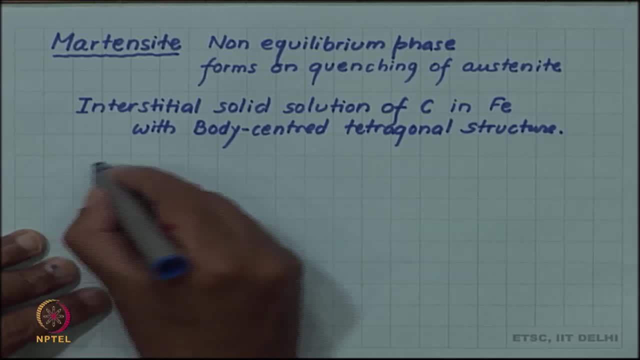 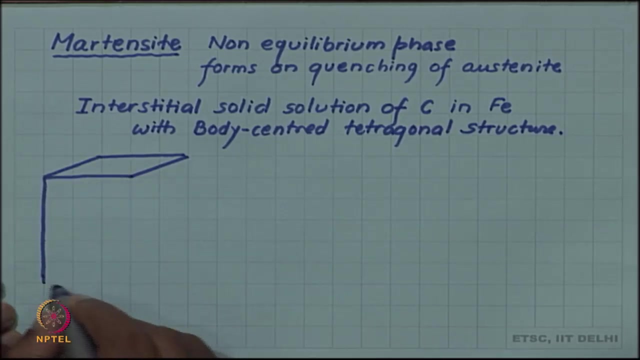 for us called by body centred tetragonal we mean the unit cell of body centred tetragonal will be like body centred cubic. Only thing is that one of the axis, the c, 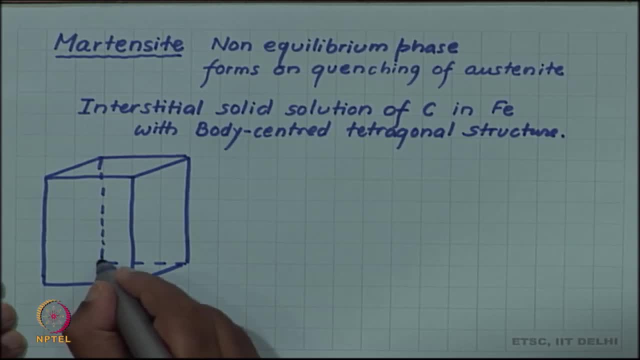 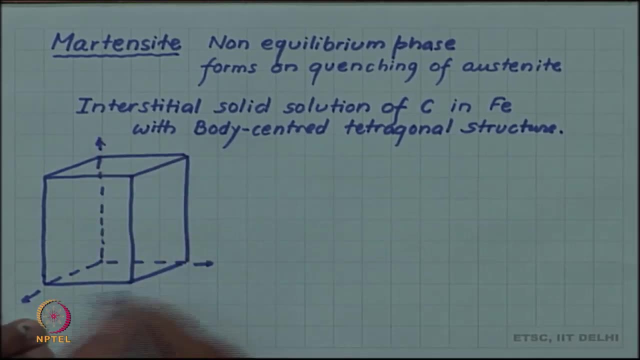 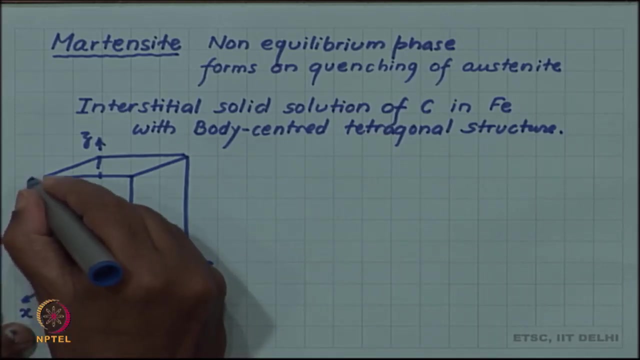 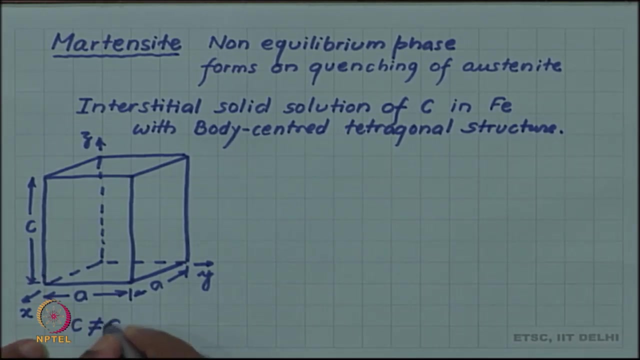 axis will be longer than the other two edges of the unit cell. So this length along x and y, these are a, But this length will be longer than the other two edges of the unit cell. So this length along the z axis is c and c is not equal to a. if c was equal to a it will be cubic c, not 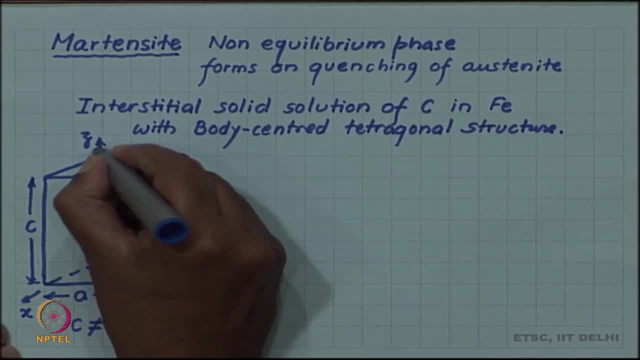 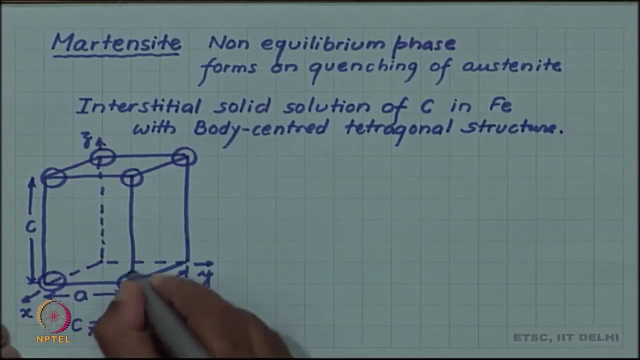 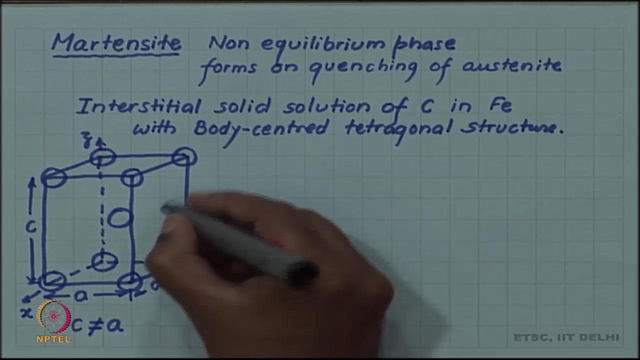 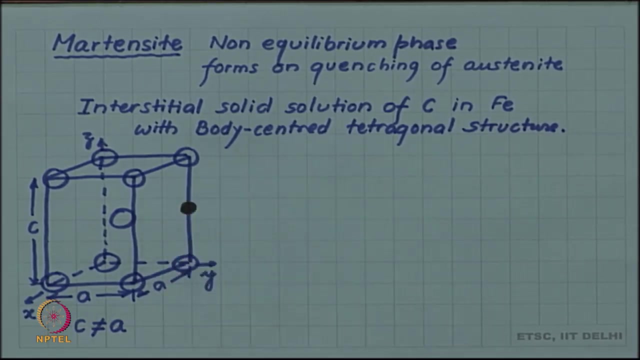 equal to a gives us tetragonal. The ion sets at the corners and the body centre, because this is body centred, Body centred cubic. and carbon finds its location in the middle of the edges of the c axis- This is ion and this is carbon. And the c by a, this is c and c is equal to c. this distance, 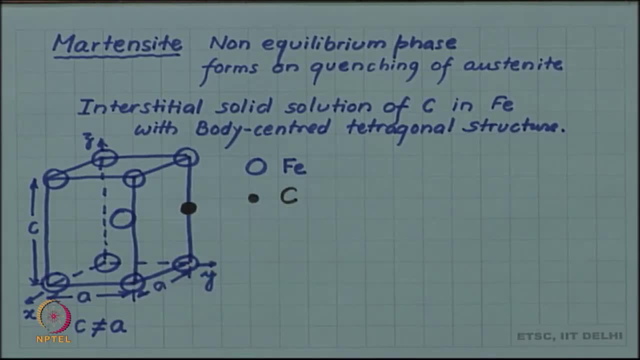 that is, the δ is equal to distance: c per 분 of the surface. This is the dipole value. Now it all different sections. each of these is different, So it is two sides clicking on one, and this issta is fairly different points. holding everything together: Moving. 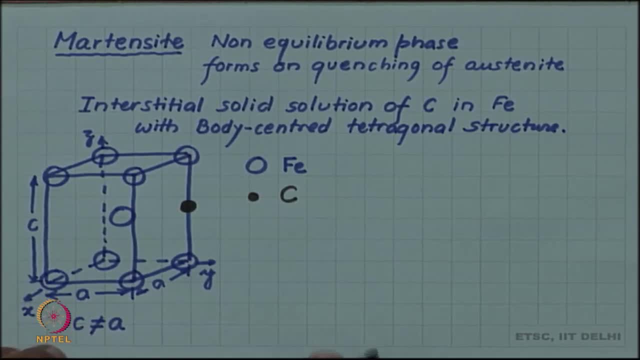 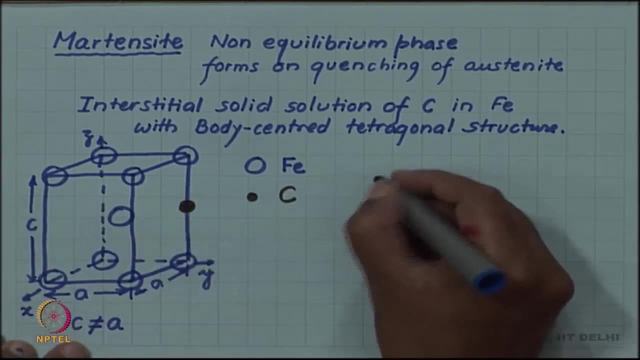 on to other SA. So this is altogether three hairs, saying an element all over the body, and the C by A ratio is not very high. So remember that if C by A becomes equal to 1, if C by A equals to 1, it is no more tetragonal, it becomes body centered, cubic. So that is. 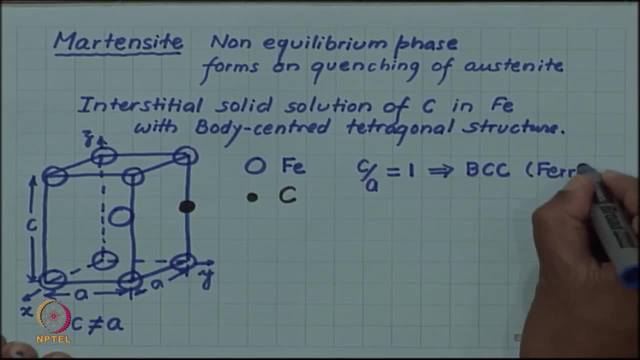 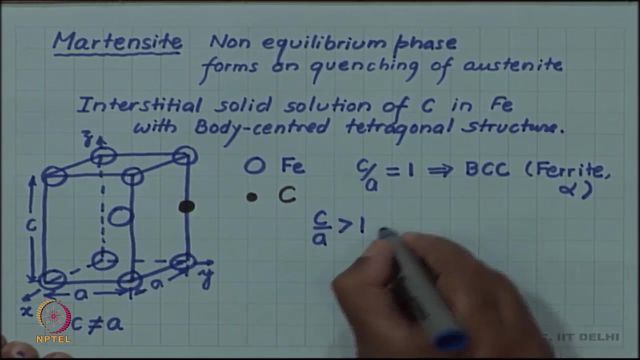 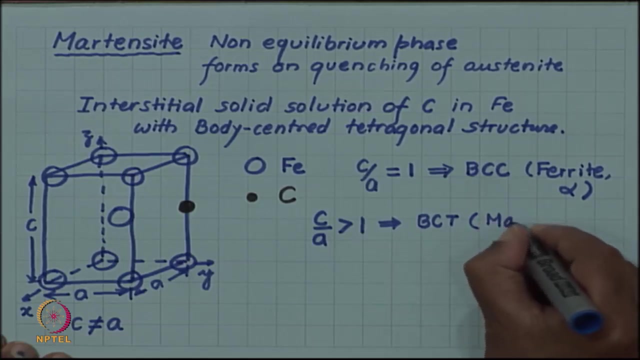 what is your ferrite? you use the symbol alpha for ferrite, but if C by A is greater than 1, then it is body centered tetragonal, and that is what is our martensite. I gave the symbol M for this, but because of its relation to ferrite, you can see it is. 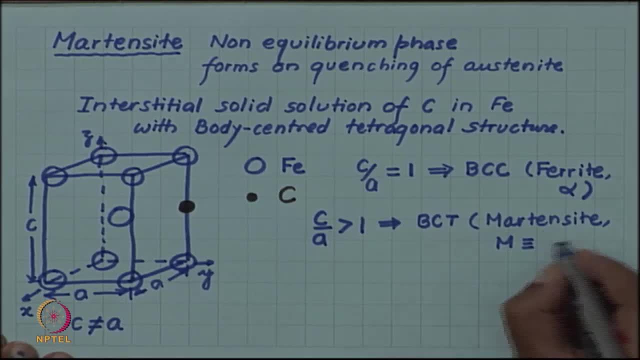 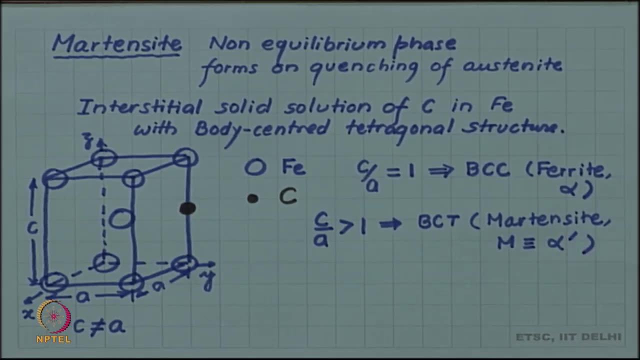 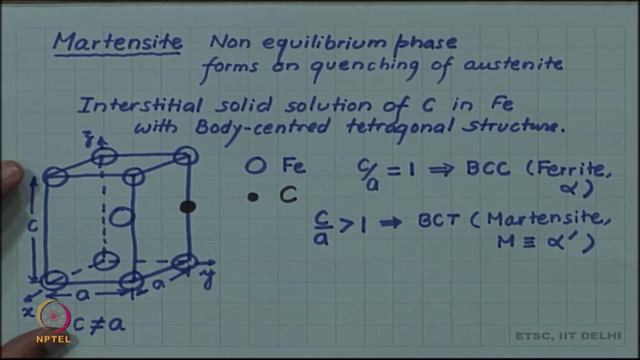 a slight distortion of ferrite which will give you martensite. So sometimes it is also have a designation alpha prime. So alpha is BCC, alpha prime is body centered tetragonal. This crystal structure is very hard and brittle So it is important in terms of its property. 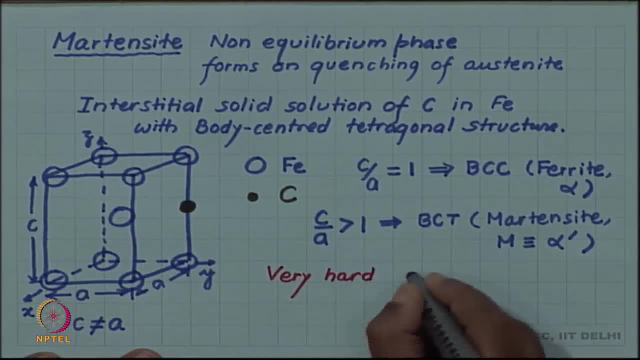 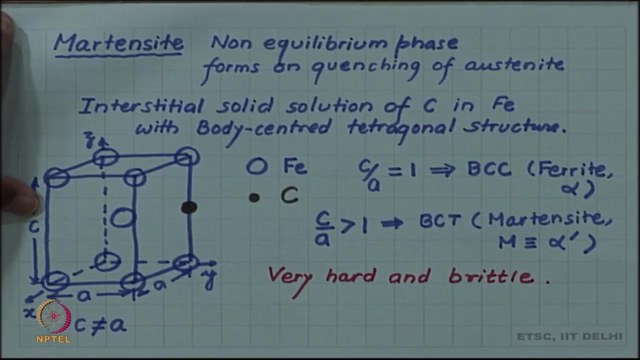 is that it is very hard, which is a good news, but it is also brittle, which is a bad news. So very hard and brittle. We already discussed about the ferrite, So we will discuss about the ferrite. So let us see how to make the ferrite. So here we. 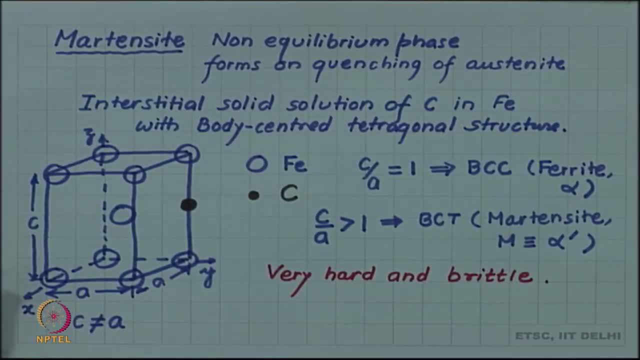 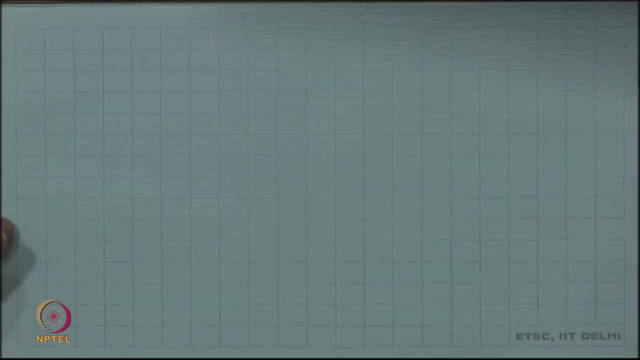 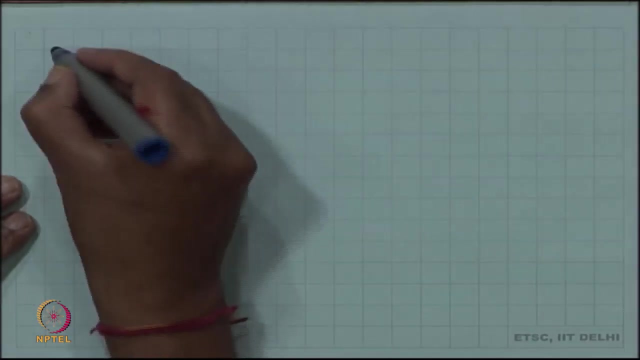 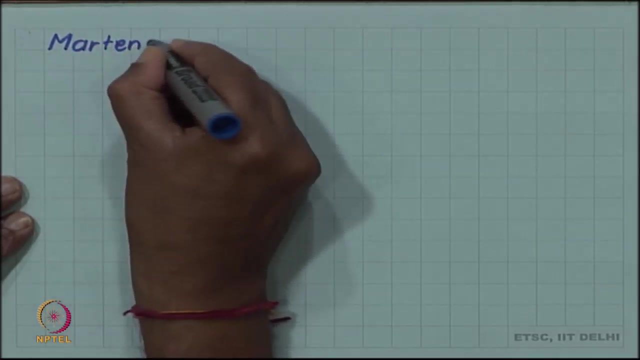 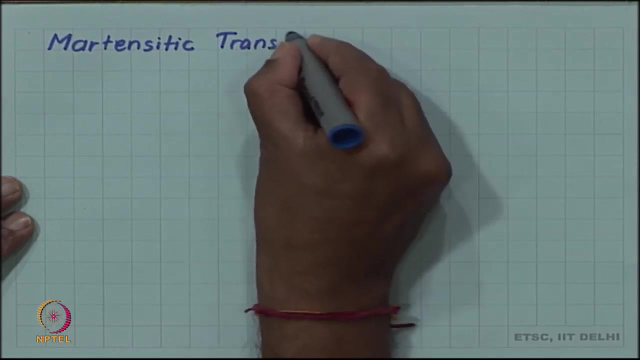 already talked about some differences in the way austenite transforms to martensite, So let us note those differences. So this is a very these differences are very important, so much So that all such transformations are labeled as martensitic transformation. 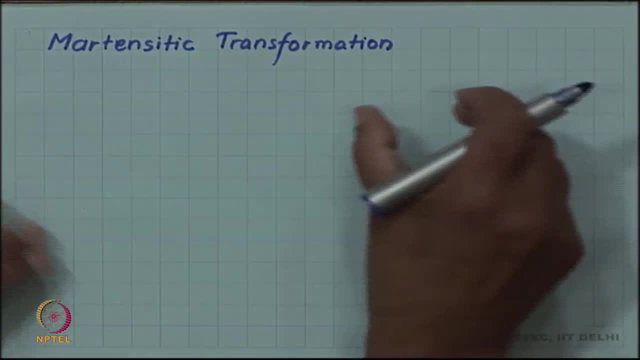 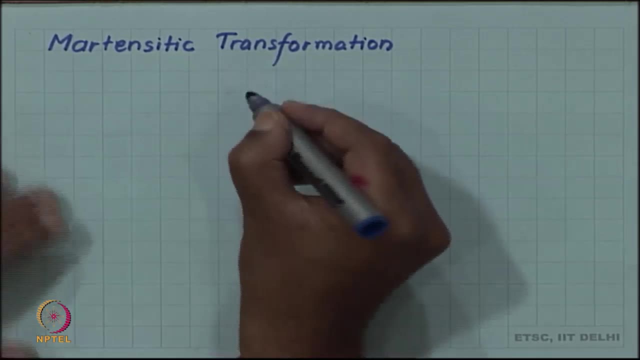 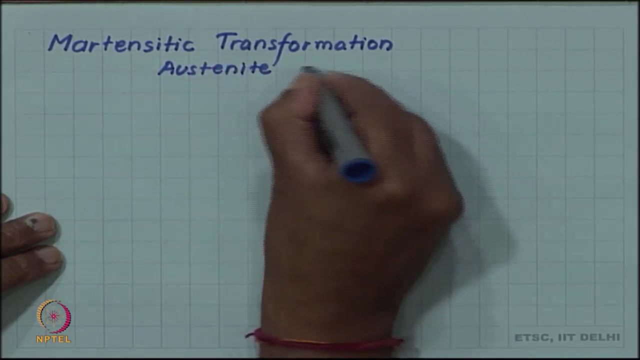 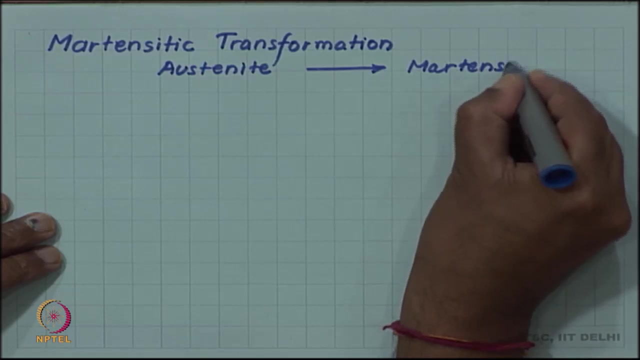 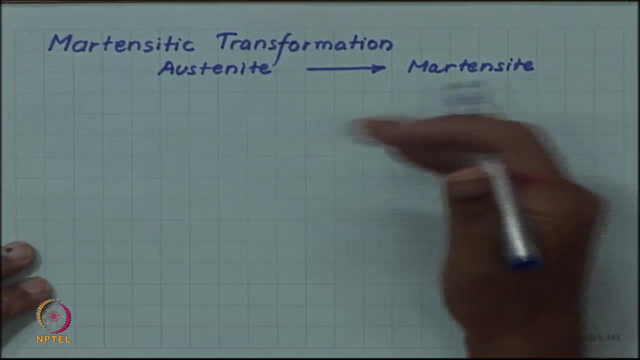 martensitic transformation, of which the transformation of austenite to martensite is a prototype. So austenite transforming to martensite is known as martensitic transformation, but it has several characteristics and any transformation which shares those characteristics will always 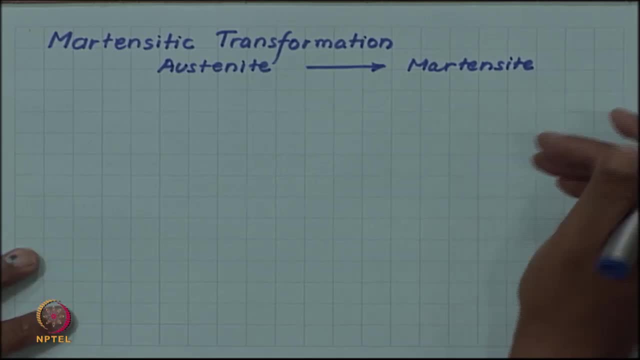 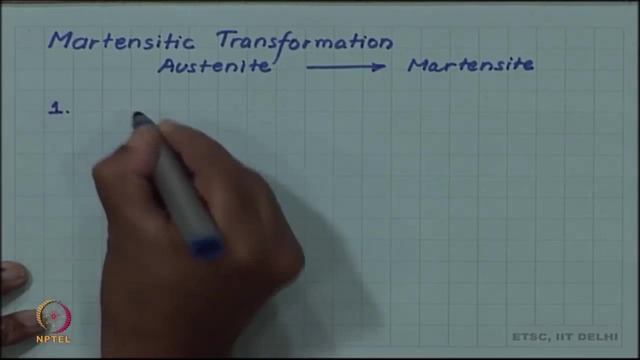 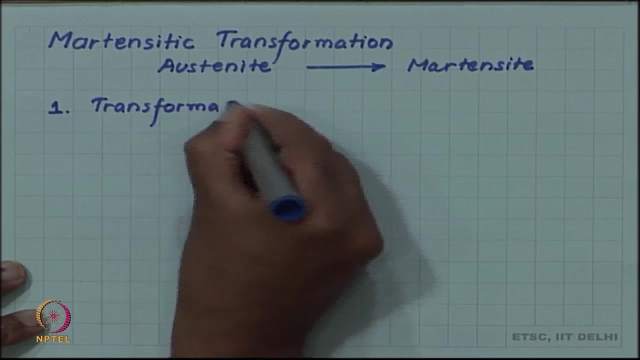 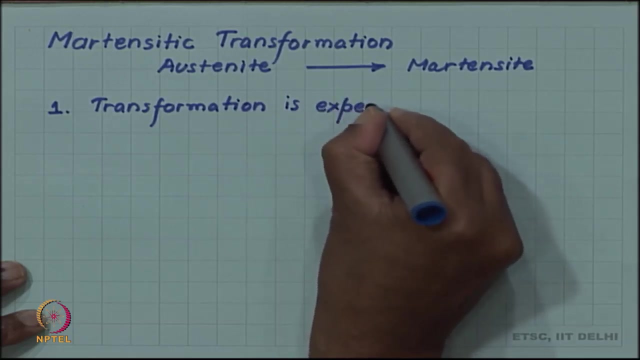 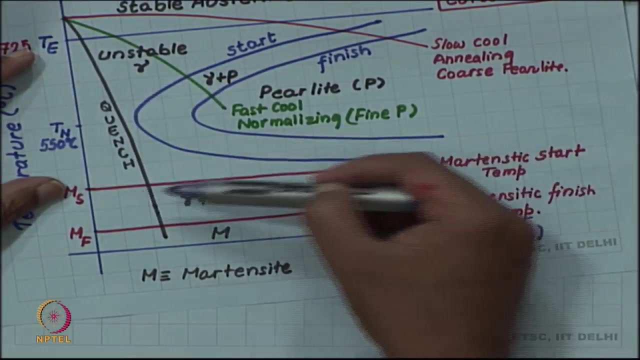 also be called martensitic transformation. So what are those characteristics of martensitic transformation? First of all, the transformation is extremely rapid and that is why it is possible to have the transformation even on rapid quenching, which is not giving much time for transformation to happen. So the transformation itself is extremely. 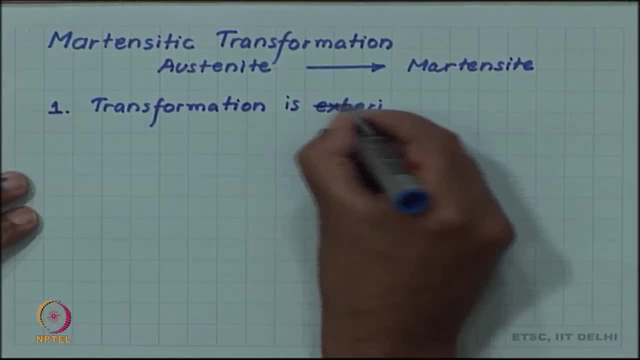 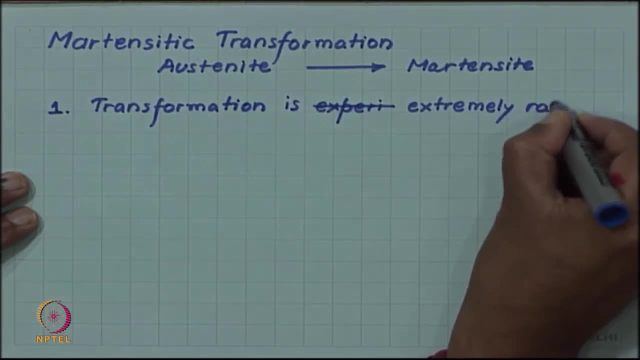 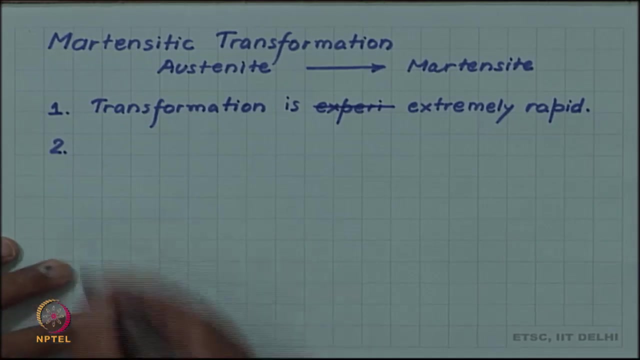 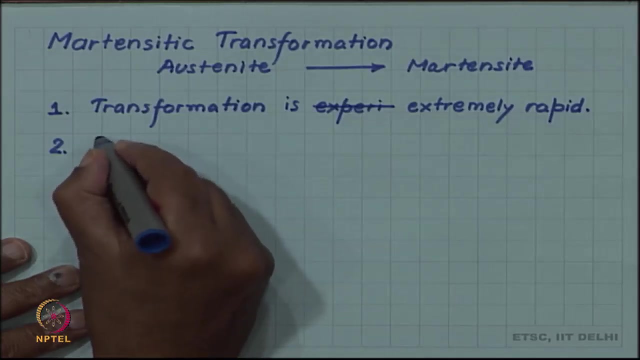 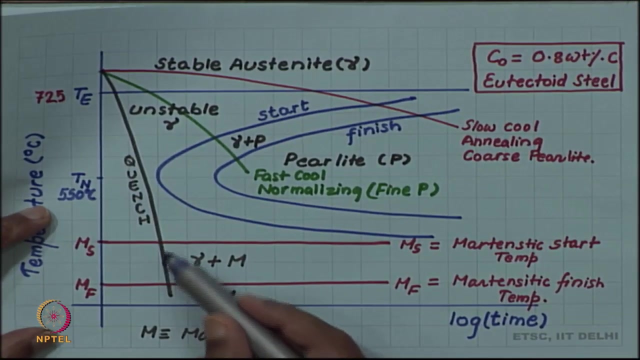 rapid, sorry, transformation is extremely rapid. it completes in no time. And since it completes in no time, we see that the rate of transformation does not depend upon temperature. So amount transformed, as I indicated to you here, amount transformed only depends upon the temperature at which you have reached. So at M S the transformation. 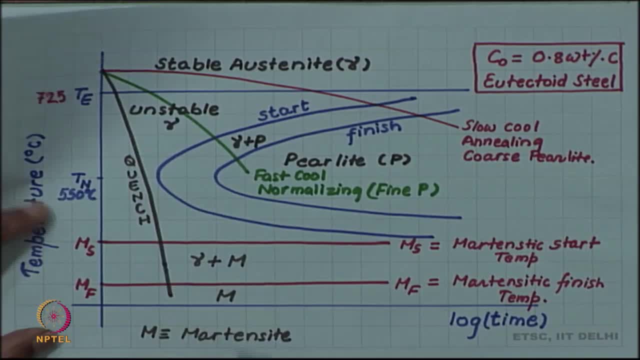 has just begin and then gradually it increases and at M F it completes. So amount transformed. So at M F you have reached Now this gives you a following one. This might be the second term. okay, This is another example of this transform. So you see that the transformation, 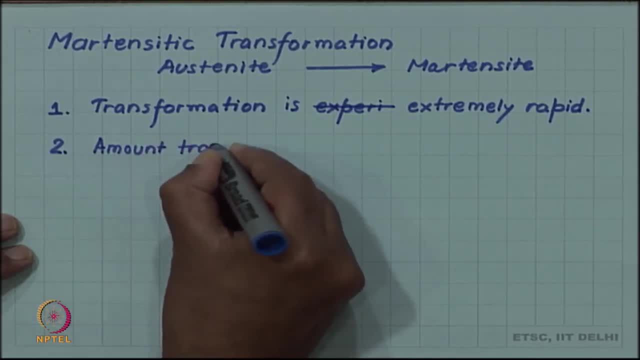 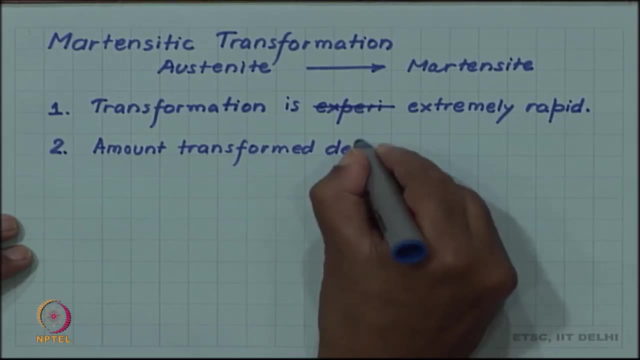 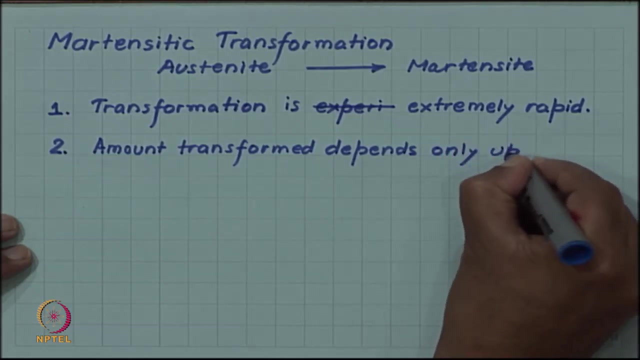 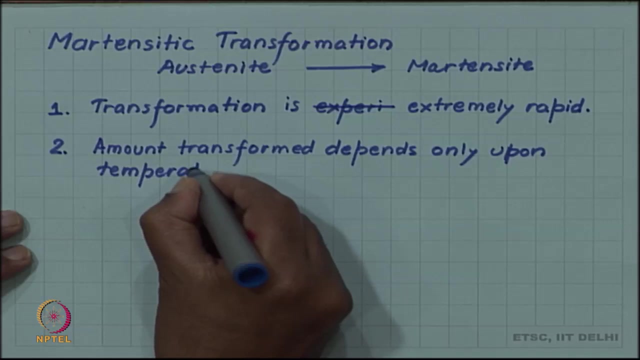 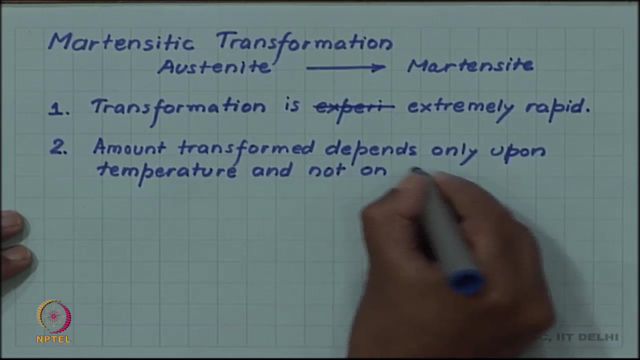 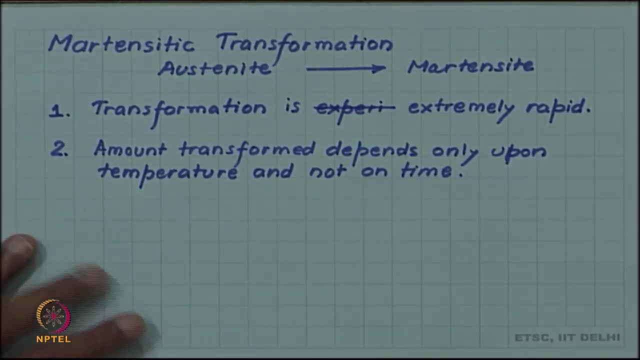 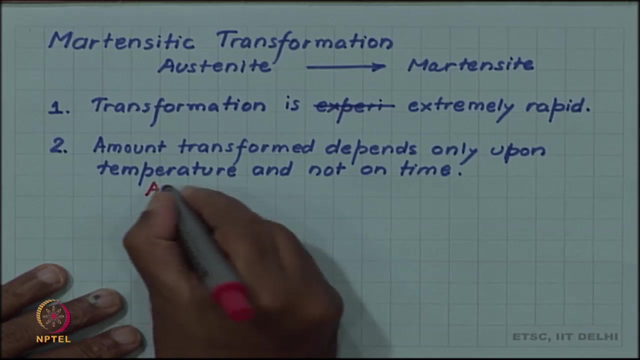 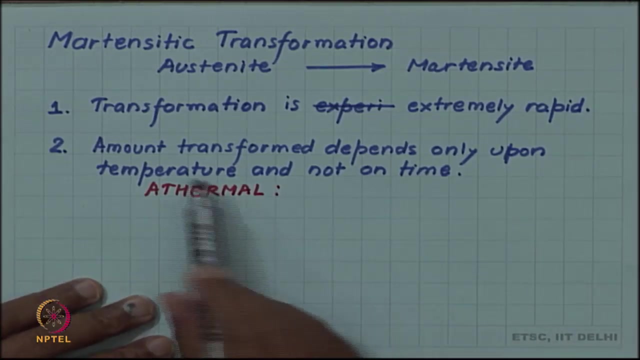 It depends only upon temperature And not on time. to emphasize this, sometimes a phrase- a thermal- is used and such transformation are called a thermal, And by a thermal we mean it is little confusing term to use because, you see, amount transform depends on temperature but not on time. and we are using the term a thermal, which means 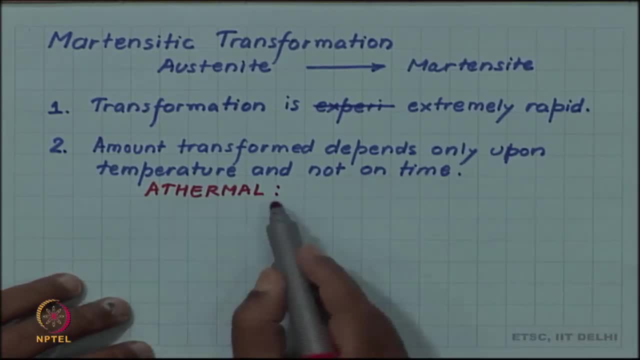 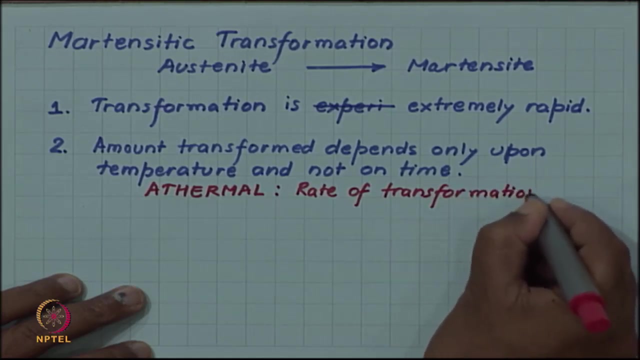 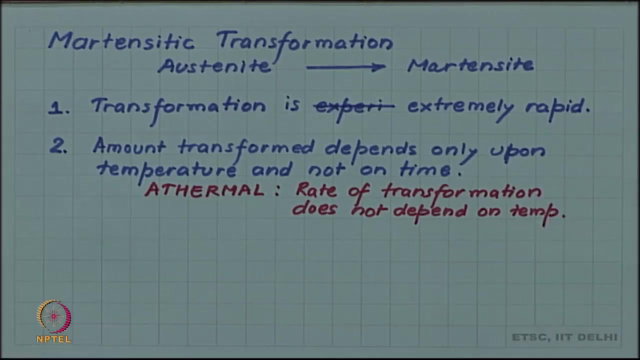 that it is independent of thermal effect. but what is independent is the rate of transformation. So a rate of transformation Does not depend on temperature and that is why you did not have the C curve. in the case of C curve, you can see, the very existence of C curve is indicating that the rate of 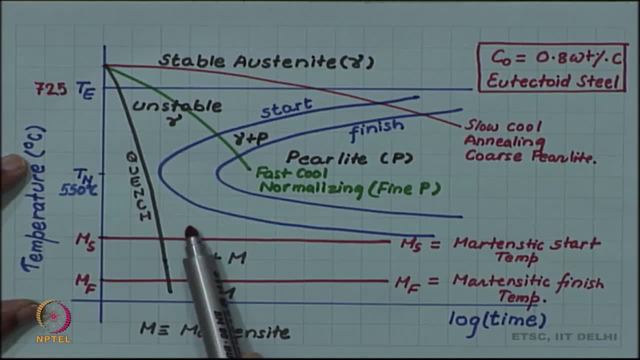 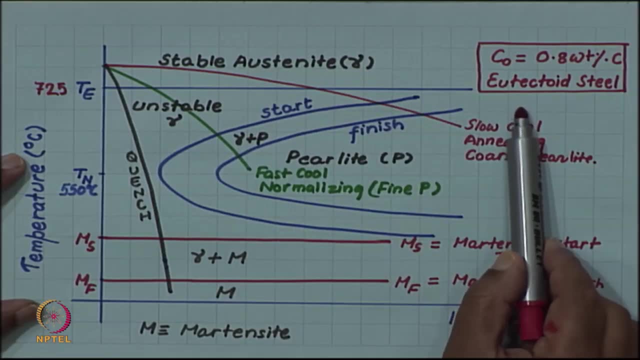 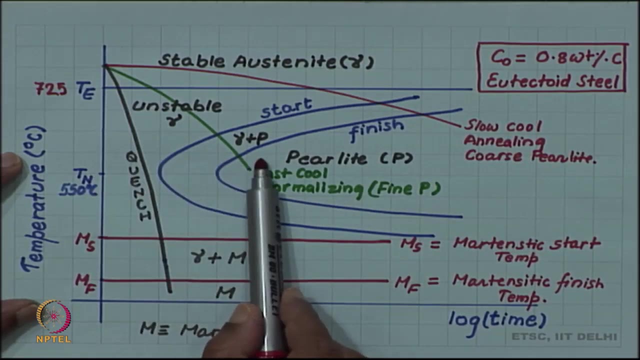 transformation are strong function of temperature. So just below T e the time required for transformation to pearlite. It is very high. the rate is very slow. but close to the nose the rate is very high and the transformation to pearlite is very rapid. 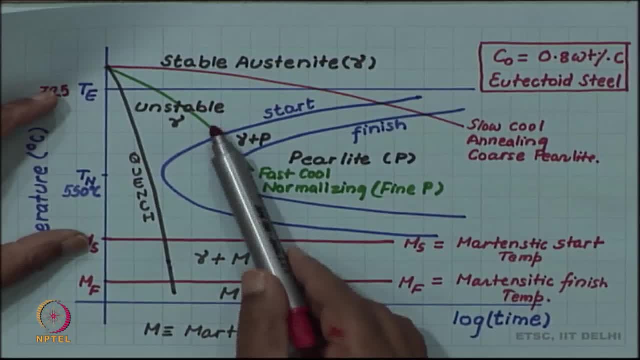 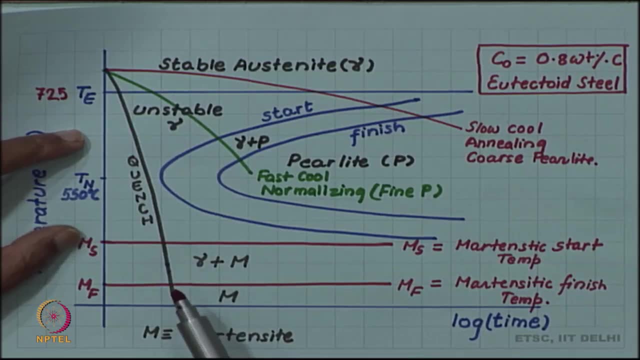 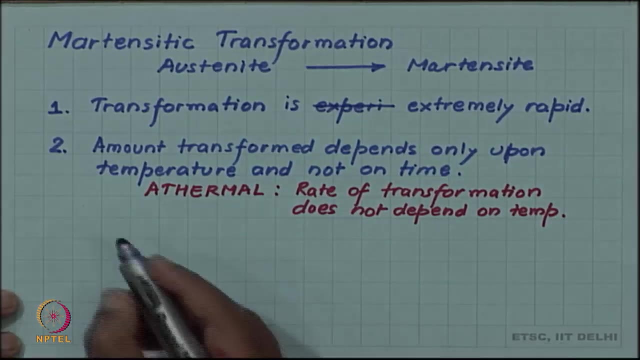 So the C curve is an indicator that the rate depends upon temperature. but here the horizontal lines for M s and M f are indicating, and the absence of C curve is indicating that the rate does not depend upon temperature. So this is called an, a thermal transformation. 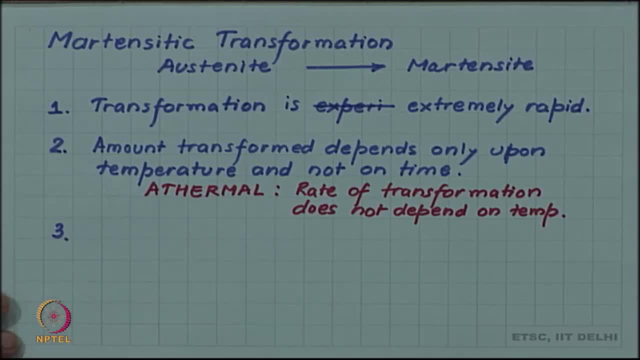 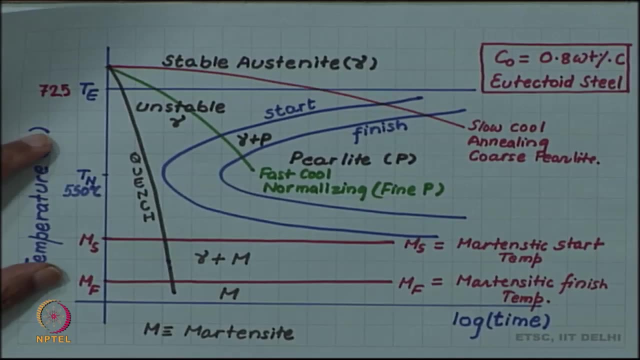 Thank you, Thank you, Thank you, Fine, Thank you. Another important characteristic of the transformation is that the composition is not changing. So if we had eutectoid steel and if we are cooling it very fast, there is no time for. 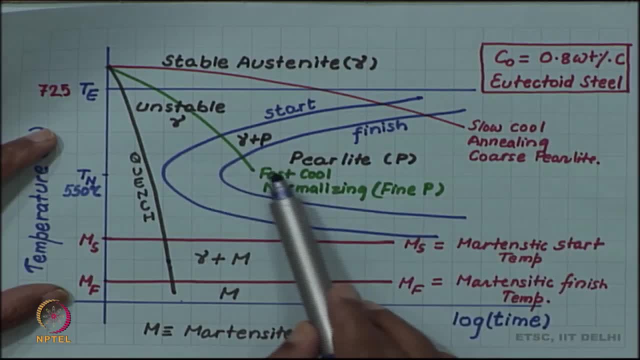 composition to change. So in pearlite, when pearlite formed, remember, although we started with 0.8 weight percent carbon, The pearlite is consisting of ferrite, which has very low carbon- 0.2 weight percent carbon- and cementite, which had very high carbon- 6.67.. So enormous composition change happened when austenite. 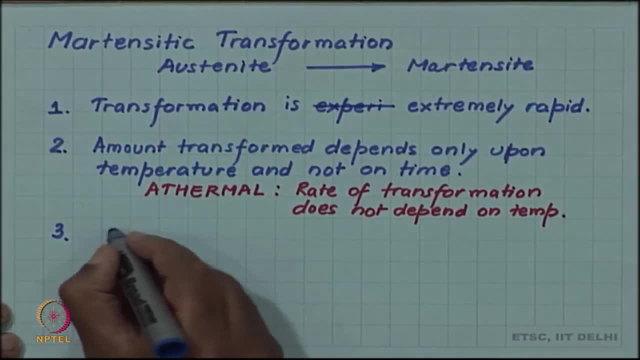 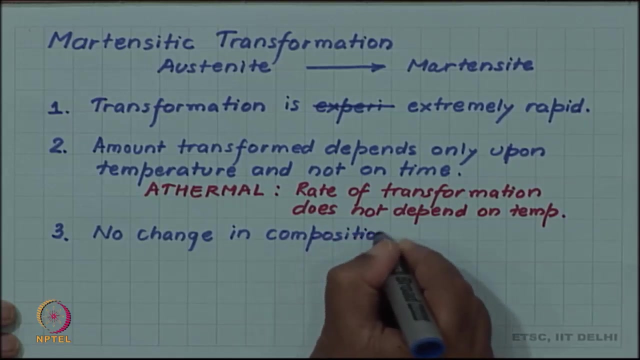 transformed to pearlite. no such thing happens in martensite, so no change in composition. This is linked to the fact that transformation is very rapid. since composition change is not required, transformation can happen very fast. If composition change is required, diffusion will be required and time will be required, and diffusion rates are dependent on temperature. 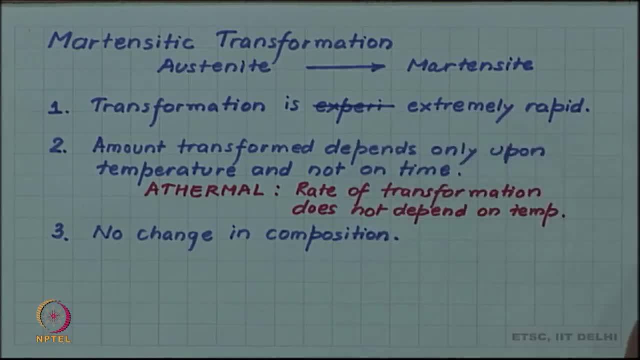 so the rates will depend upon temperature. So these facts are not all really independent but are interlinked. So there is no change in composition. sometimes this fact is also stated as by saying that the transformation is diffusion less. When we say diffusion less, you can see that. 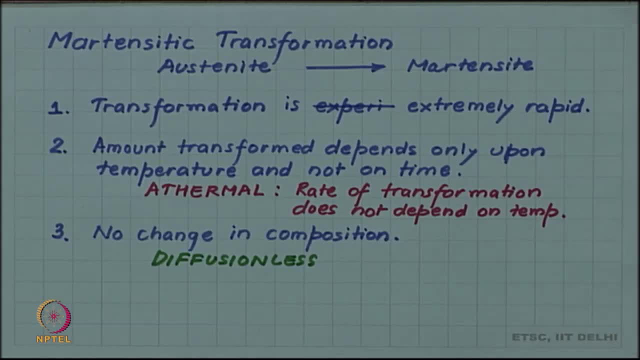 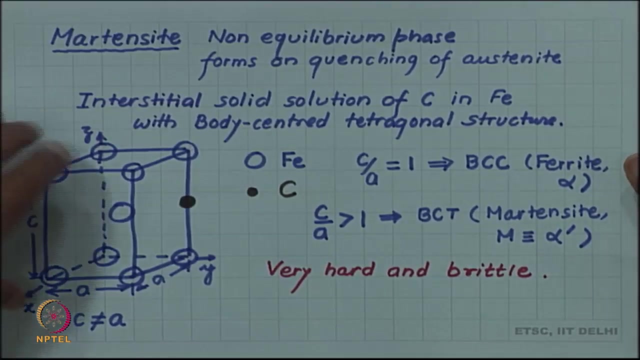 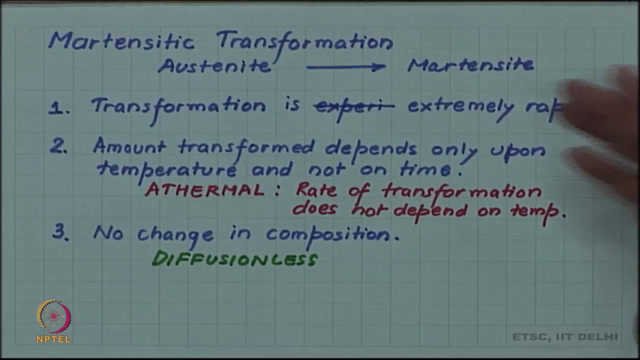 the transformation is requiring a change in crystal structure. but when we are saying that the transformation is diffusion less, for crystal structure to change, atoms have to move, As we will show how that is possible. so very little movement of atom, less than 1. 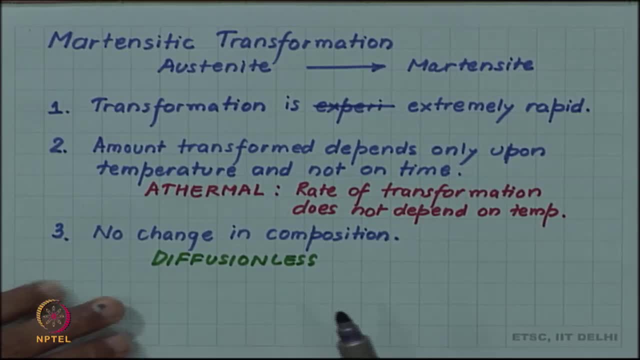 complete atomic jump, let us say, will lead to the transformation, whereas diffusionless we mean in diffusion we mean long range atomic transport. So by this diffusion less we mean that there is no long range diffusion atomatic Alejandro. atomic movement.